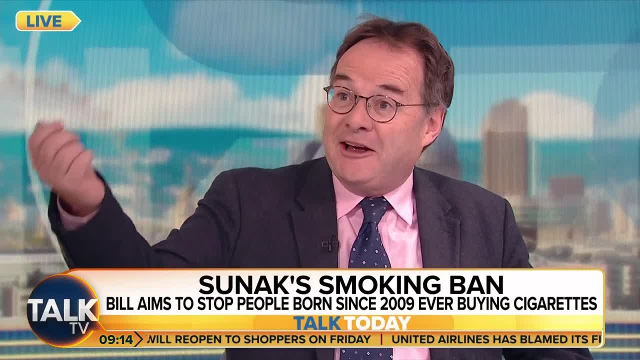 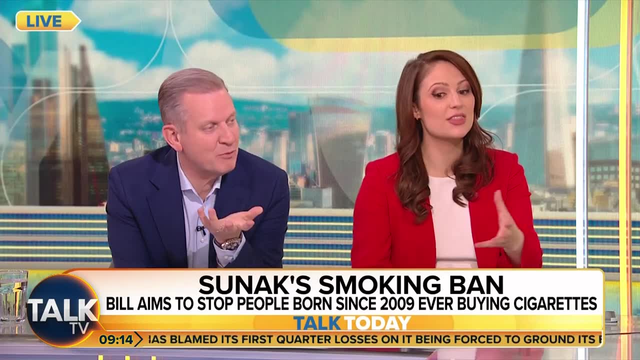 standing outside your WH Smith Giving a fact to an 81. waiting for the 81-year-old to come out with their box of. But isn't the point that it significantly reduces? It will significantly reduce. I think it'll happen with evolution. 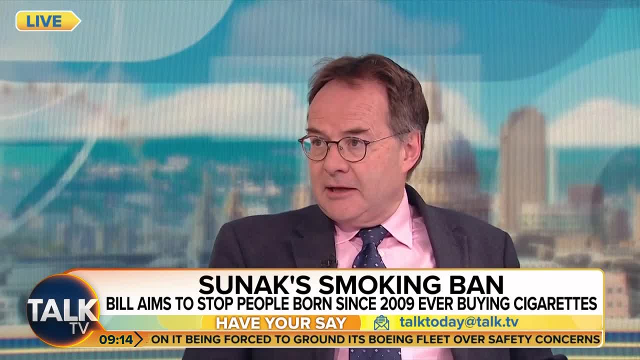 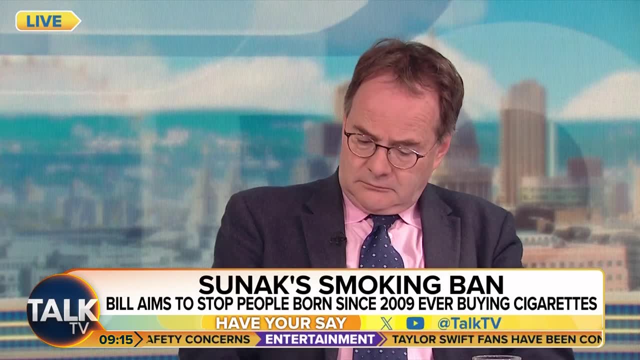 the numbers? Well, it already. It's speeding. It's acting to speed it up, isn't it? I've been saying all morning: We don't look back at the indoor smoking ban in 2007 and go, oh, I wish we hadn't done that. It did, It was effective. 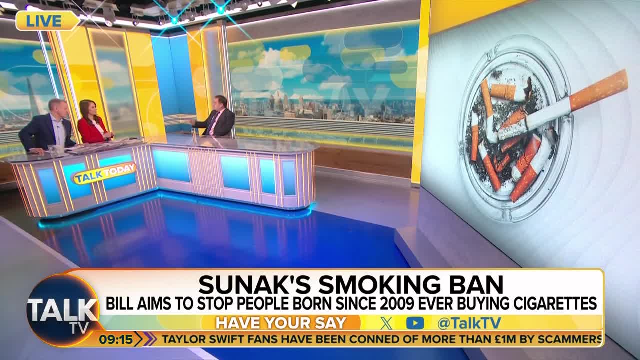 We were saying, Quentin, we used to be able to smoke on planes. My thing about it Tubes been said in the morning as well. yeah, On the tube. Yeah, you used to have ashtrays on the tube. 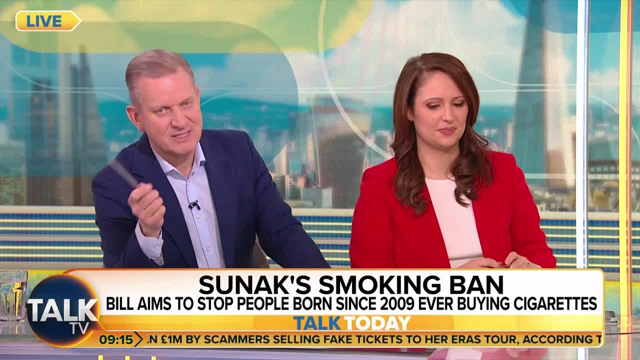 And look why I'm the King's Cross. I personally think they should. I'm not against. I think people should make their own minds up. I don't doubt the health issues. We should certainly be looking at what's inside vapes. 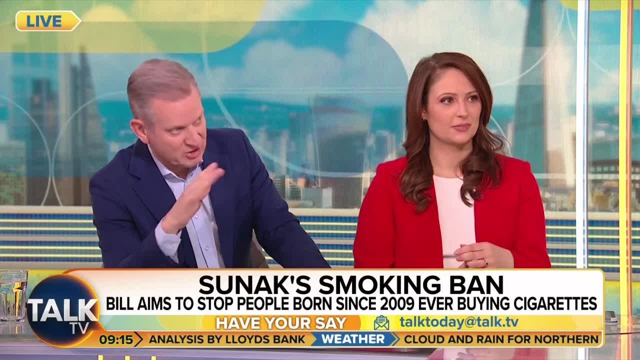 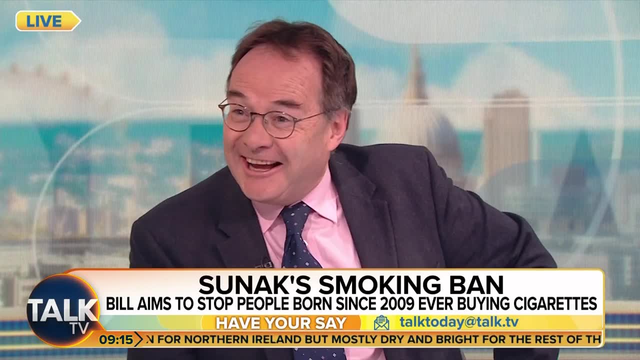 The doctor said to me, when I They don't know what's in there, those things at all. I'm not condoning smoking, but those vapes can and will be very dangerous. I want to move you on from smoking. He's banning your talk on smoking. 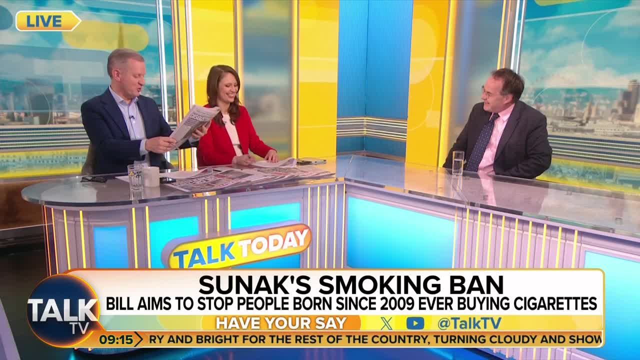 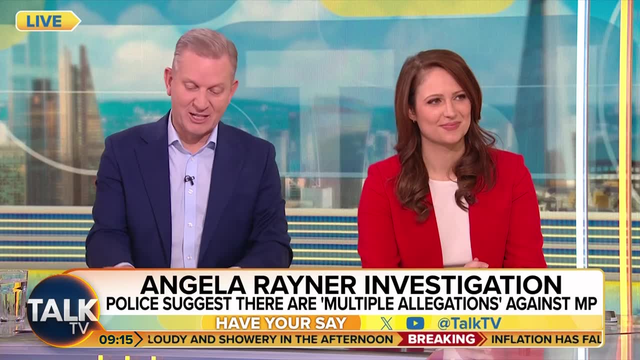 I thought perhaps there was someone behind me, Because I will not let this story go. I keep being pushed back. Angela Rayner, Quentin, can you please explain to me about a woman who I quite like? Angela Rayner, I like her too. 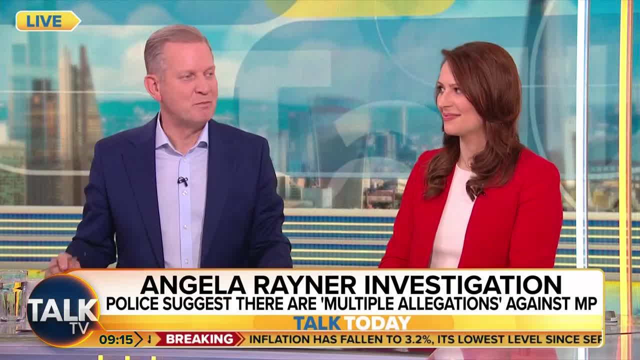 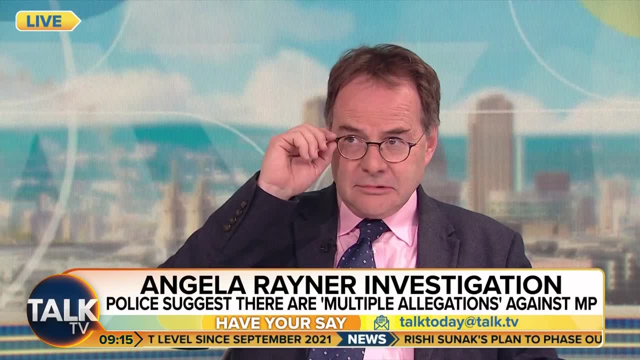 She's a little bit of joy and ballsiness and otherwise tepid beige. House of Commons. However, we've known about the houses. I had somebody yesterday who went. well, it's only three £3,000.. The Tories owed 500.. 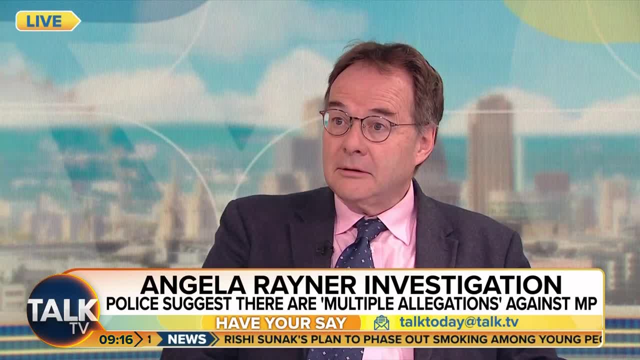 Not about that. it's about if you're going to be in a high state of office. have you lied or not? What I don't understand- and you would know these people- is if you're telling the truth, Aranj, get the papers out and give them. 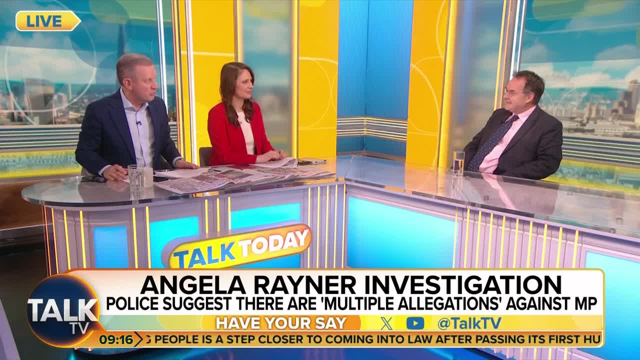 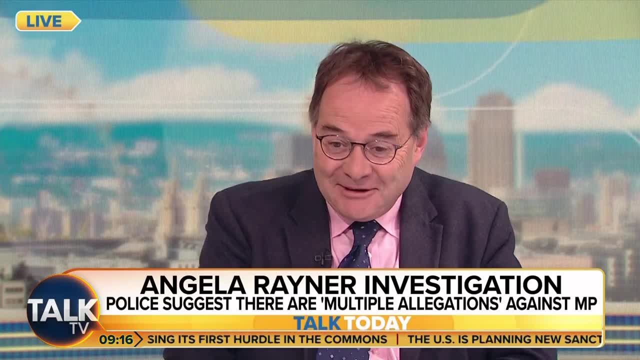 And all these people say: well, she hasn't been asked yet. Give them to the newspapers and show that you're innocent, right, If she's got the papers- I mean, I personally, my own personal bookkeeping is in such disarray I'd never be able to find the papers. 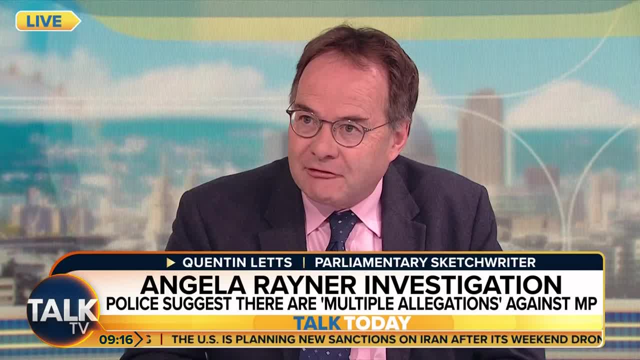 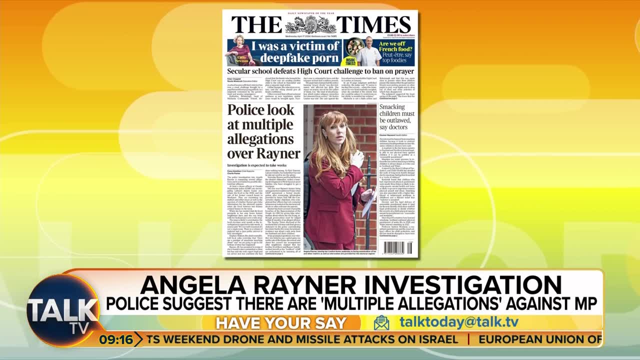 But the thing about it? she's a finger-wagger, isn't she? She's always telling other people off, and she's always had a terrible go at Boris for being unhygienic in his morals, And now it turns out she herself might have been. 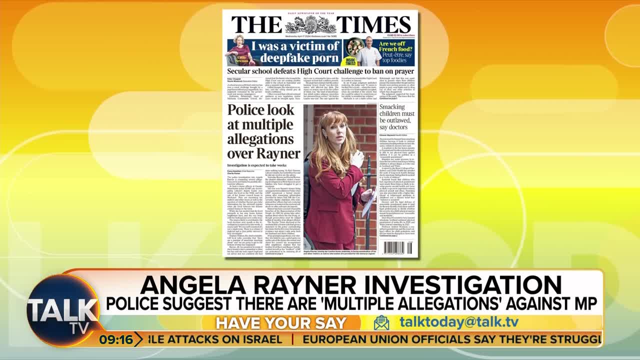 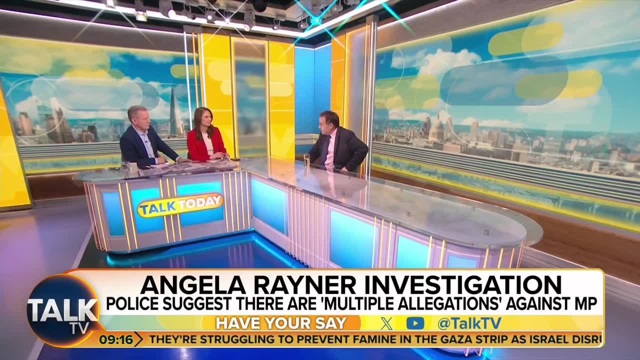 a little bit careless in some of her bookkeeping. So I mean my personal feeling about this. we have, all of us, tried to play a canny game on tax matters. Speak for yourself, Quentin. Well, I bet you employ an accountant, don't you?